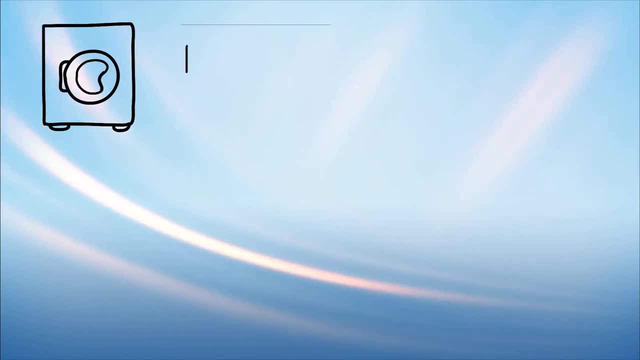 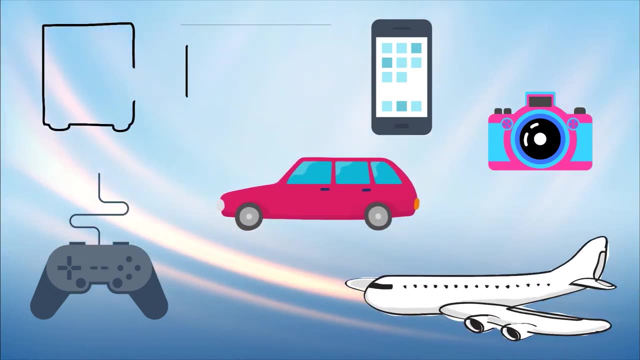 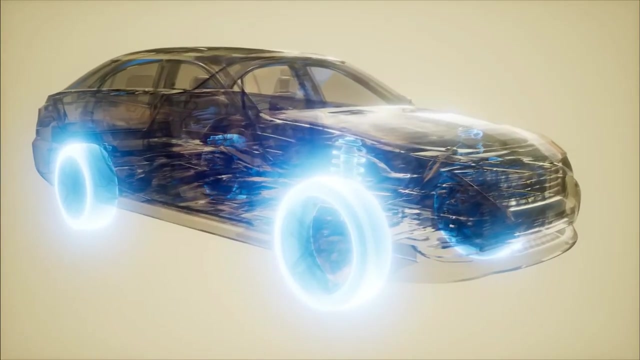 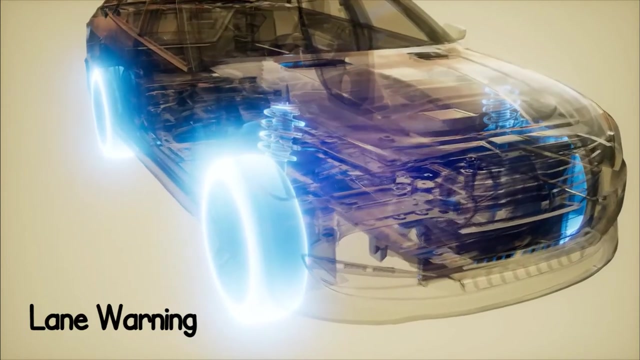 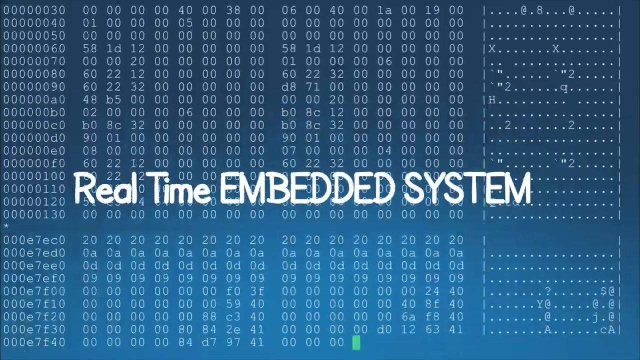 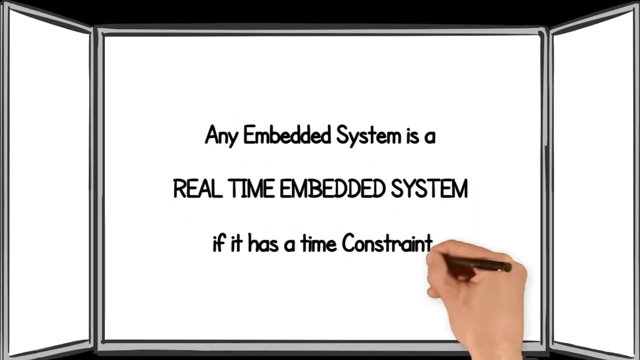 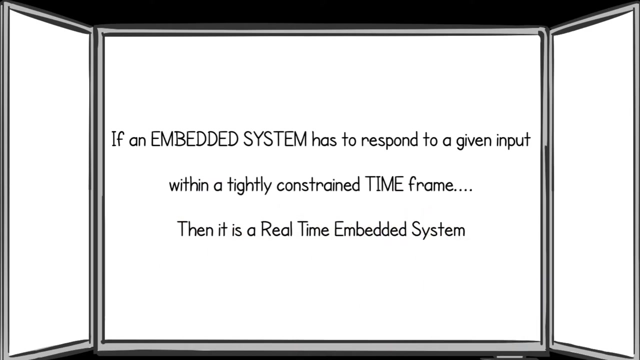 Embedded systems are everywhere: in washing machines, microwave ovens, mobile phones, digital camera, video game consoles, automobiles, aerospace computers, artificial start things up, Testblocks, Hack, CRUISE MOTOR TRACK TRACK to respond to a given input within a tightly constrained time frame for 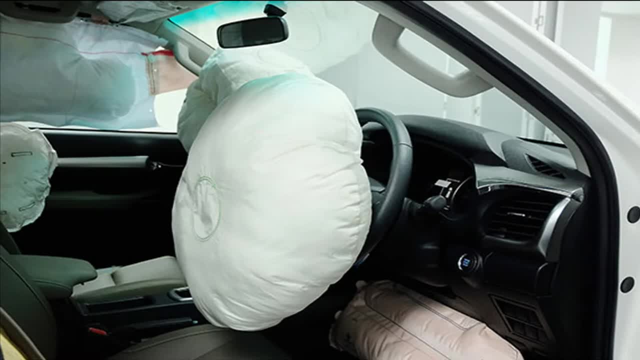 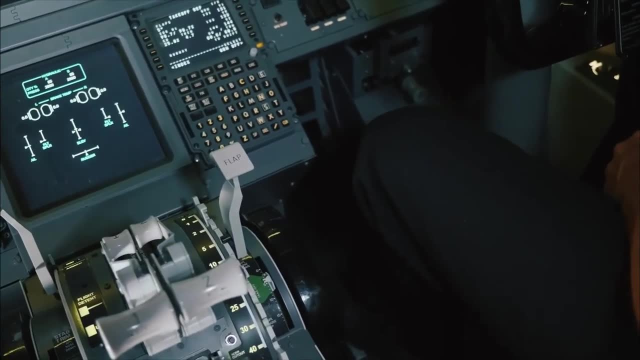 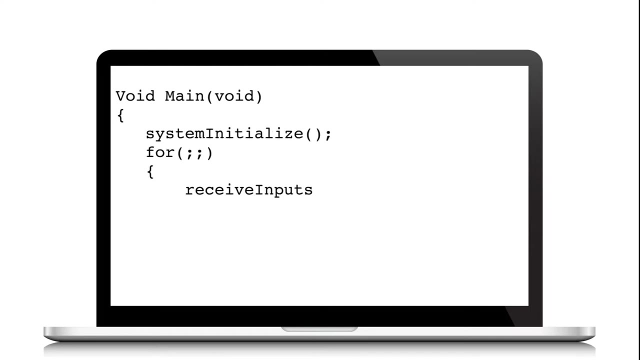 example, an airbag system in a car can be considered as a real-time embedded system. a flight control system in an aircraft is a real-time embedded system if an embedded system is as small and as simple as processing some external inputs, maybe sensors, and controlling some output devices, maybe one or more. 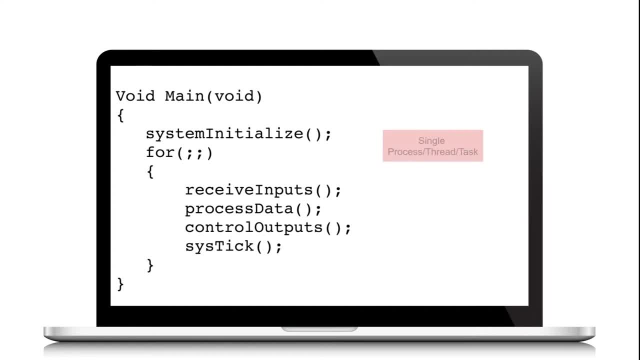 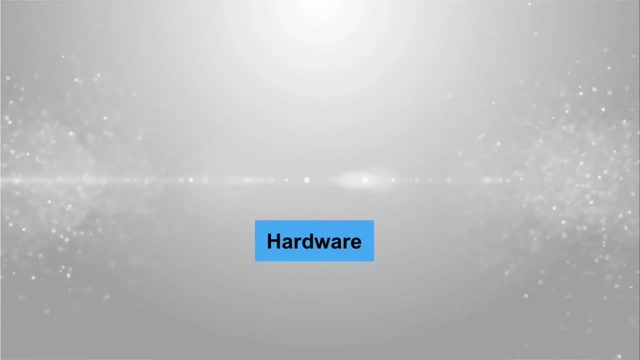 actuators and this can be handled using a single process or a task within the application software, then there is absolutely no need of a real-time operating system, RTOS and such a basic embedded system can be layered as hardware, I O devices, device drivers, which are nothing but embedded software. 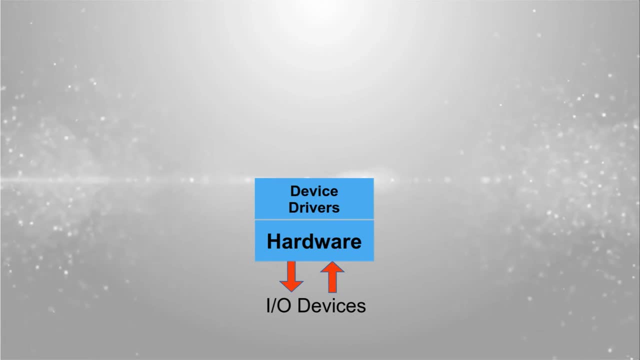 modules to operate the hardware devices, and then an application software which processes the different inputs and commands the outputs based on the application need. now, if your embedded system is a little complex and you would like to manage it with the optimum use of its resources, then you will need to. 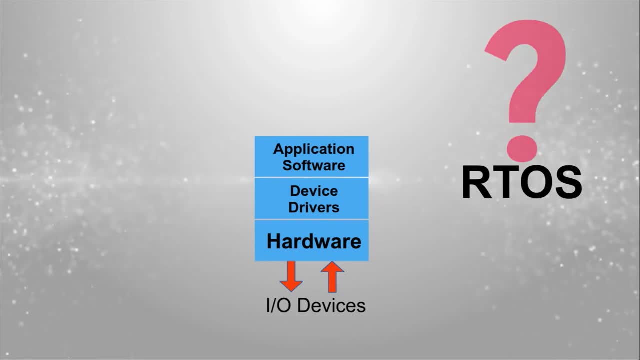 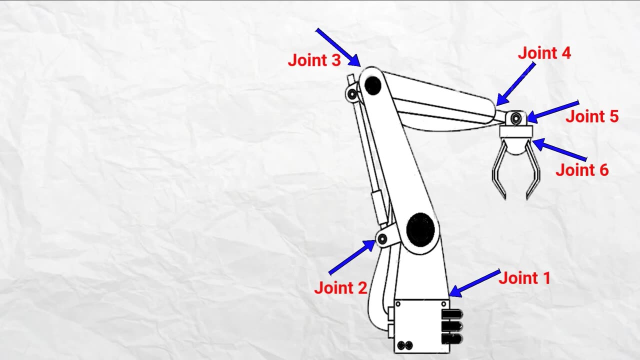 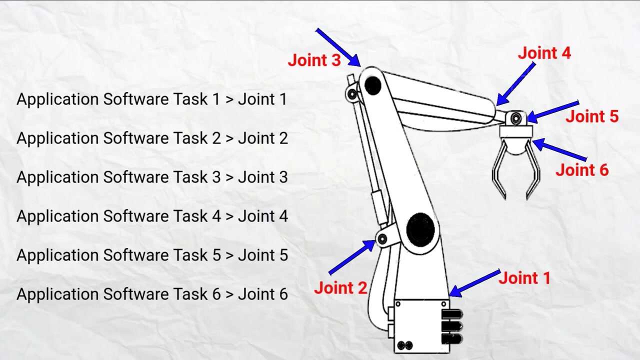 include a real-time operating system in your embedded system. take this example: a robotic arm having, let's say, six joints, which are also called as access, which needs to be controlled accurately. in this case, you would be required to separate the application functionality to multiple tasks, each task, or a thread controlling each of the joint or access.